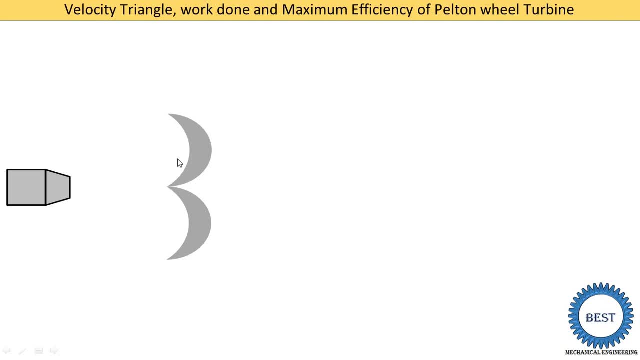 strike on the splitter And after the striking jet is moving from this, both the spherical bucket and water is outlet from these parts. So the water coming with the velocity v1 and it strike to plate. So we draw this one line and its line is indicating the absolute velocity of a jet v1 and its land is a to c and it is a land a to c. So 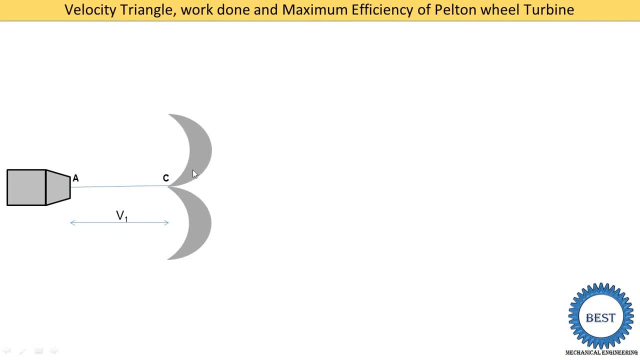 a to c is indicate the absolute velocity v1.. Now, after striking by, this bucket is start to move with velocity you. this bucket is start to velocity you, so on this line we are required to draw the velocity you. so velocity of the bucket is always less than the velocity of a jet and this bucket 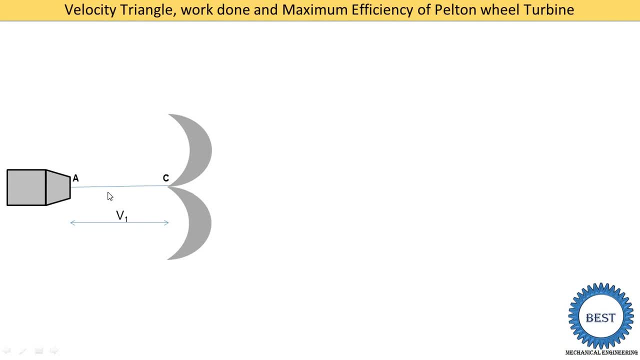 is moving in a, x direction. So on this a to c- some parties- we indicate the velocity of a bucket, u1, and it's drawn as the a to b. so this a to b line is indicate the velocity of the bucket because it is also in horizontal direction. so we draw on the same line of the v1 now remaining velocity. 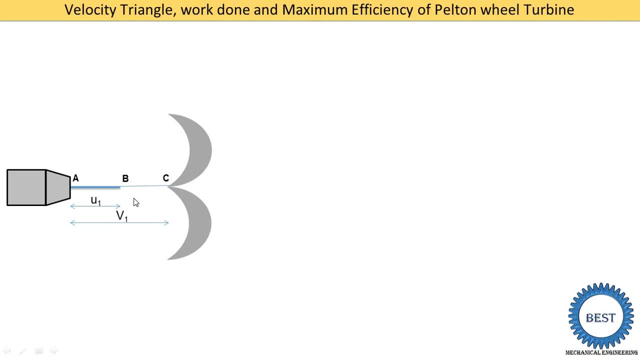 is the relative velocity. relative means with respect to the other velocity, so velocity of z with respect to the bucket, so this known as the relative velocity. and relative velocity is v1 minus u1, so a to c is v1, a to b is u1, so remaining part is bc. so this bc part is known. 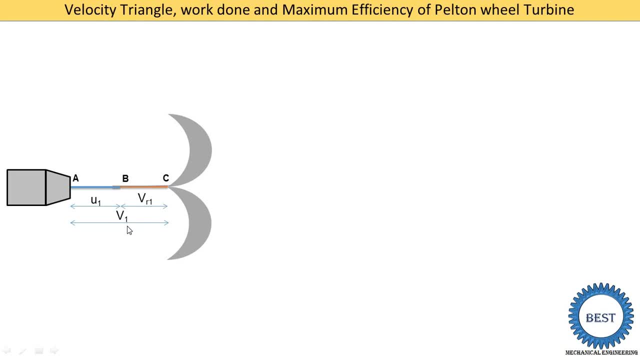 as the relative velocity, vr1. so vr1 is equal to v1 minus u1. another example is that if you sitting on this bucket and you see the velocity of a jet, then which velocity you see in it is known as the relative velocity. after that the water is moving. 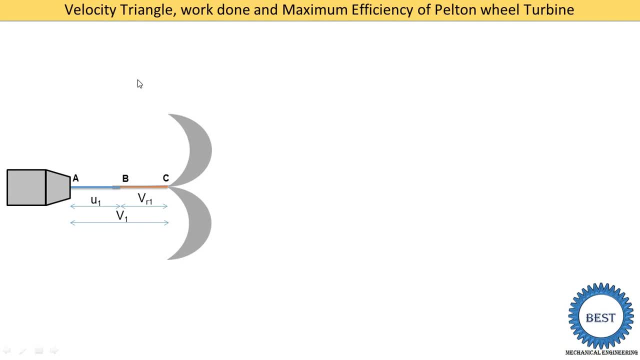 you see, the water is moving with the surface of this bucket and exit from here at the velocity v2. so for that here the angle of deflection is given, and on the basis of its design. so first we draw the angle of deflection line, and this angle of deflection is denoted as the phi and is 180 degree line, so 180. 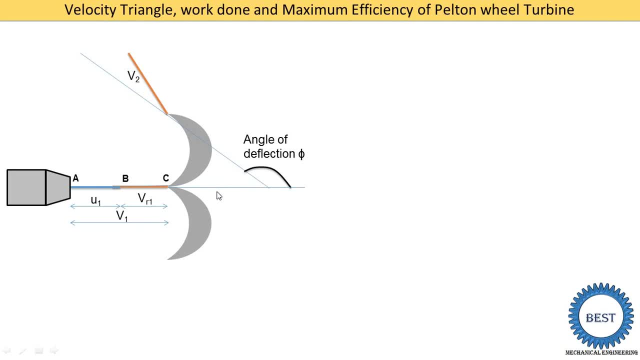 minus angle of deflection. then it's give us the beta 2. so the water is coming with the velocity v2 and it's make an angle with the X axis. it is known as the alpha 2. so this angle is alpha 2. now v2 part it's 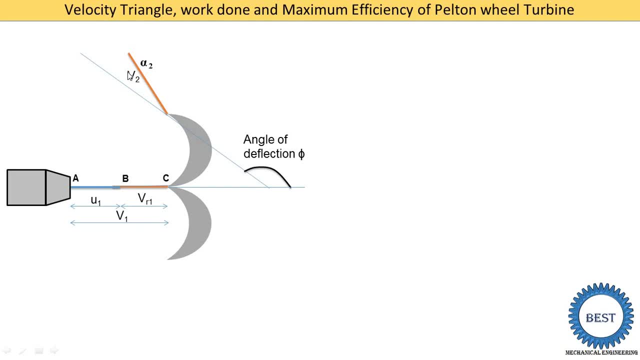 certain angle. so it is divided into two part. one is the horizontal, another is the vertical. that we already learn in a curve plate of impact object. if you don't know, there is derivation. so go to the playlists on impact object and watch the video of moving curve plate. water strike at tangential 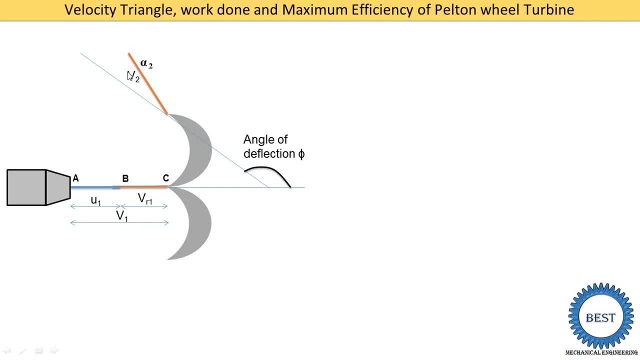 most important derivation. if you notice that that derivation then you are easily learn all other velocity triangle. so this v2 is divided in two part. one is horizontal. this horizontal part, that is green line, it's indicate the velocity of wall vw2 and this vertical part of the v2 is drawn here. 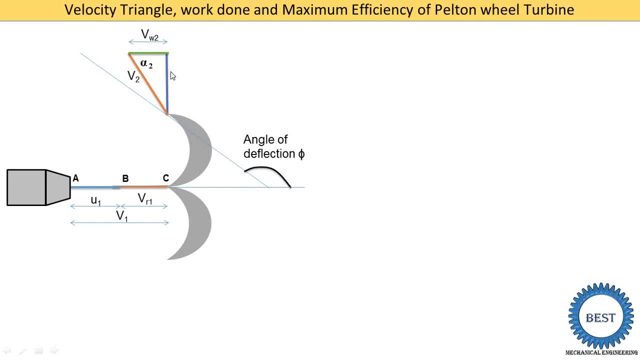 and this vertical part of the v2 is known as the velocity of flow- vf2- and horizontal part is known as the vw2. now, the another is the relative velocity. so relative velocity of the bucket, in any case, is drawn in a angle of deflection line. so this vr2 is drawn in this line, this line of 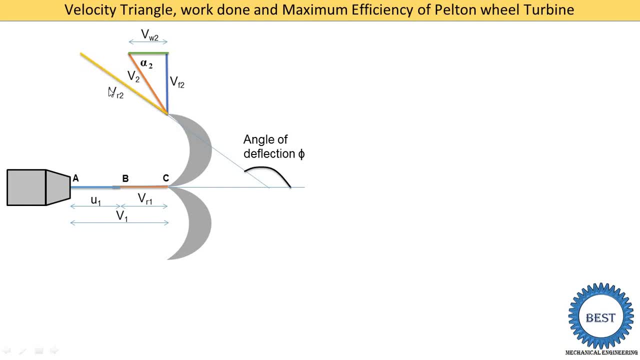 torque color is known as the relative velocity line vr2 and is we are to make an angle with horizontal axis. it is known as the beta verdad. that means angle between the x-axis and the jalylan level and when angle between the, the angle between the x-axis and the delta in the 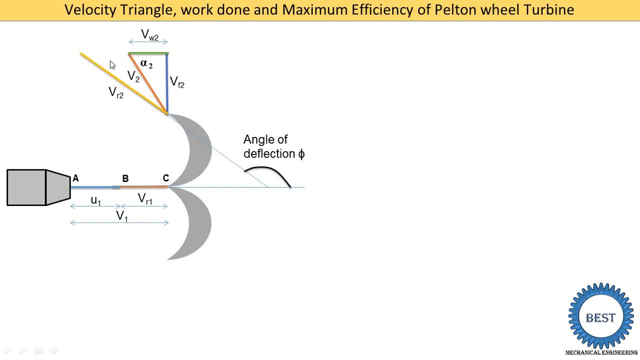 the relative velocity, or it is also known as the blade angle. so this beta 2 is also known. blade angle means this is the blade. so at the exit of the blade there is a certain angle, is known as the beta 2. now again, similar relations of the relative velocity equation is applied, that vr2. 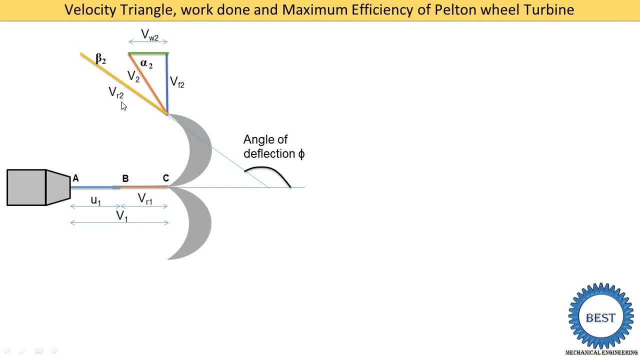 is v1 minus u1. so similarly, here vr2 is equal to relation between the u and v2, so this line is v2. so from v2 to vr2 line is drawn as the velocity of blade line, so it is known as the u2. okay, so. 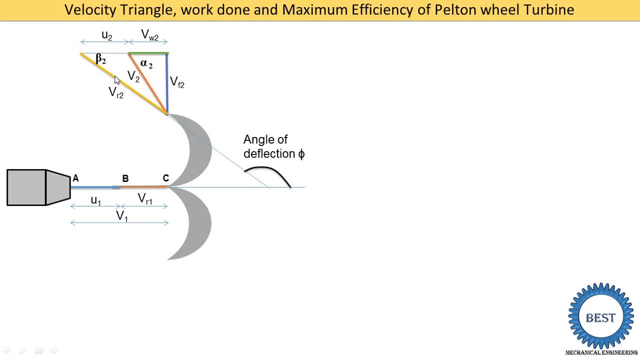 these are the very velocity triangles from a impact object. sorry, velocity triangle for pelton will turbine. next we derive the equation of work done for that. before that we learn some parameters, before that i request you to subscribe my channels if you learn something like my video and comment on the video and share with your. 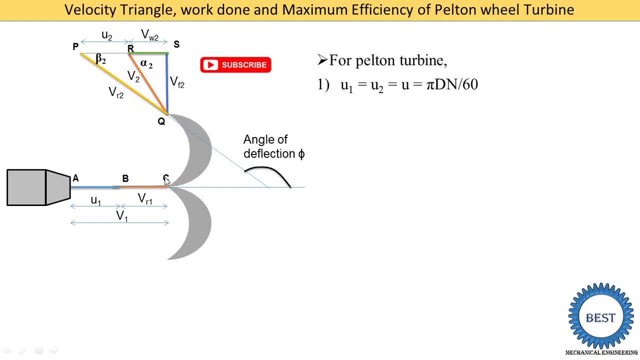 friends and family and i will see you in the next video. bye, bye. for pelton will turbine u1 equal to u2, is equal to u, is equal to pi d. n by 60 means u1 and u2, both are same. for a pelton will turbine second, alpha 1 is 0, beta 1 is 0 because in this pelton 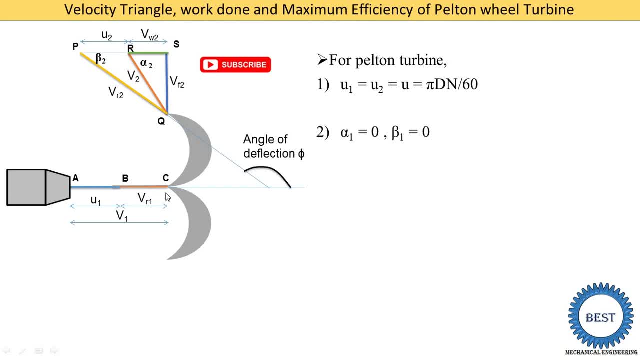 will turbine. the blade is strike in horizontal directions, okay, so angle of the nozzle is 0 and beta 1 is also 0 in this outlet, the beta 2 at the certain angle. that's why it is derived in a two parts. but in this case v1 is horizontal, so v1 is directly. 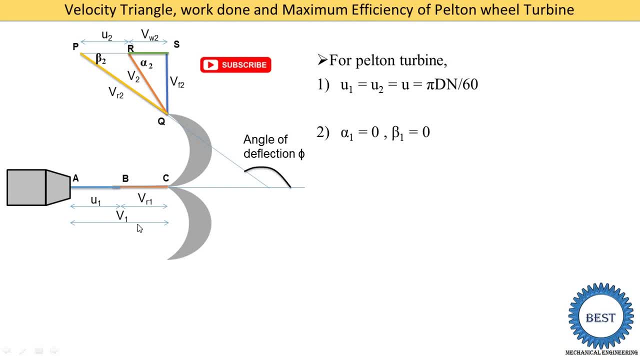 equal to vw2 because it is a horizontal, no vertical part. no vertical part means vf1 is 0, vf1 is 0, then v1 is equal to vw1. so here we write: v1 is equal to vw1. relative velocity is v1 minus u1 and u1 is equal to u. so instance of u1, we write the u. so this is the equation. 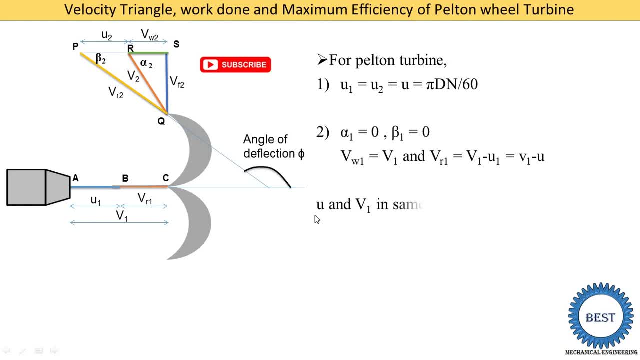 from this inlet velocity part now u and v. both are in same directions for a smooth surface of the bucket. if you assume in example the bucket is too smooth at that time relative velocity vr1 and vr2 are equal. but in some case in example there is a friction loss is given for the bucket. that 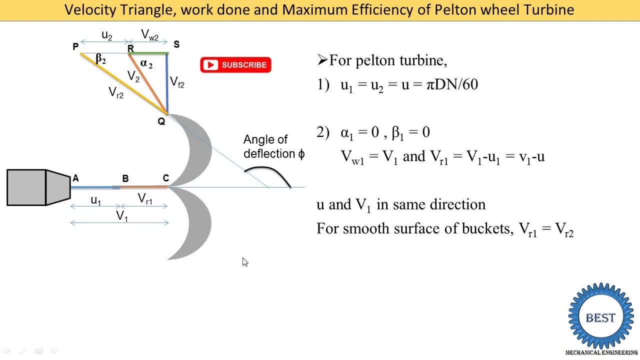 means vr1 and vr2 are not same. for that you need to find out vr2 at that time. we use the equation: vr2 is equal to kvr1 means due to friction some velocity is lost and the k is equal to blade friction coefficient in. 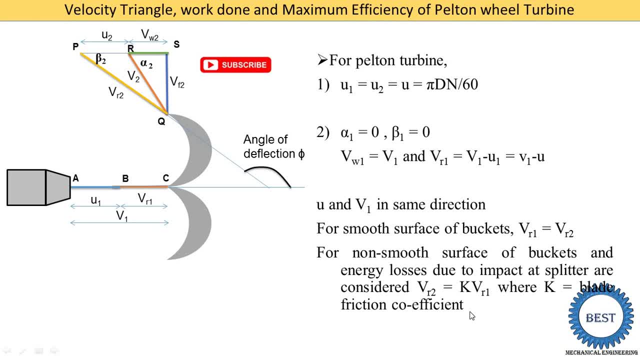 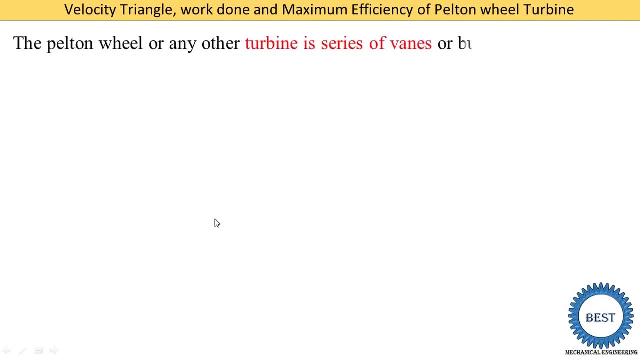 example, suppose you give the 0.85 blade friction coefficient or 85 blade friction coefficient, so you need to find out relative velocity by using this equation: vr2 is equal to kvr1. now next, how to consider the mass for this pelton wheel turbine in a pelton wheel turbine or any? 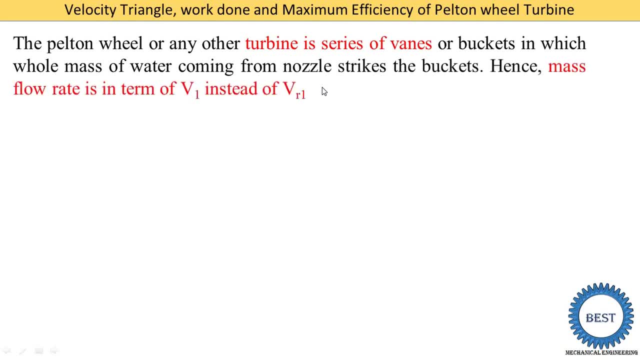 earlier turbine. that is a series of van means there is a number of bucket is there in which whole the mass of the water coming from a nozzle strike. the bucket means mass coming out from nozzle is continuously contact with the bucket, so that reasons mass flow rate is in the 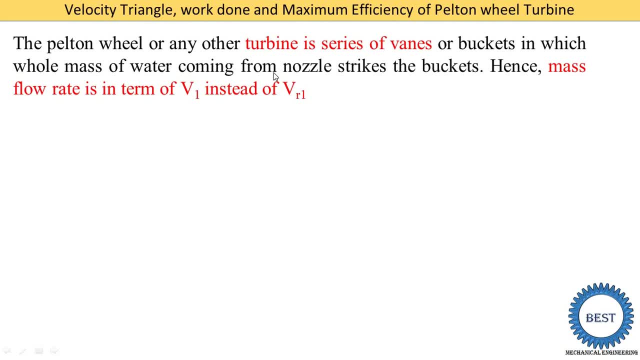 terms of v1, not in the terms of vr1. so mass is equal to rho a v1 for a pelton wheel turbine. so mass is equal to rho a v1. next we find out the force exerted by jet of water on the bucket in direction of motion. the equation of force we already find out in the case of series of plate. 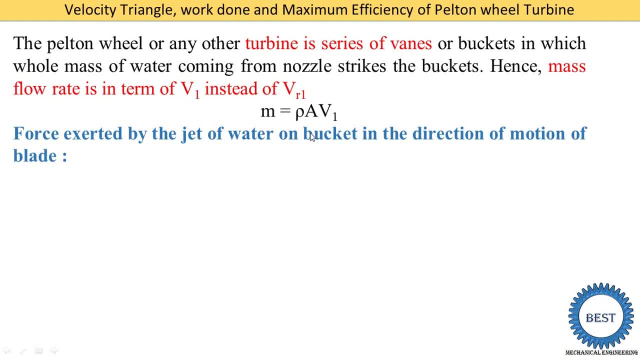 in a chapter of impact object. so we are not again derived, so we directly return the equation of fx, that is rho a v1 is equal to sorry, fx is equal to rho a v1 into vw1 plus 1 minus vw2 now, in which case we take the plus, in which case we get the minus. if you want to learn this, then go to the. 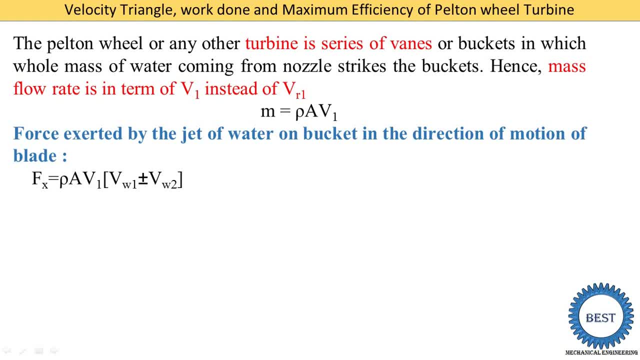 playlist or a in description and watch the video of impact object on a moving cow plate at tangentially supply. so this is a plus when the alpha 2 is less than 90. and when alpha 2 is greater than 90, then we take this minus, and when the alpha 2 equal to 90, at that time vw2 is 0. so this is the 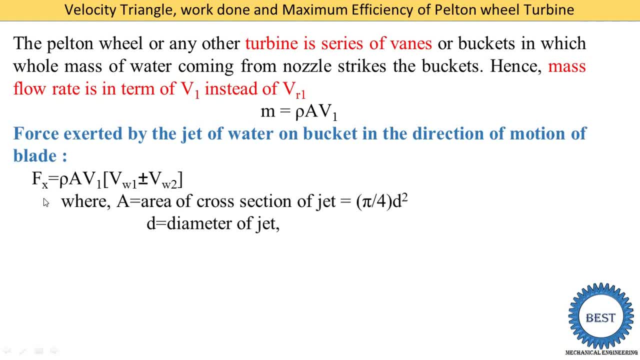 equation of fx that a is cross sectional area, pi by 4 d square. d is equal to diameter of jet, rho is density of water that is taken 1000s. next we find out a work done. work done is equal to force into distance displaced, that is, the fx into u. so this is the 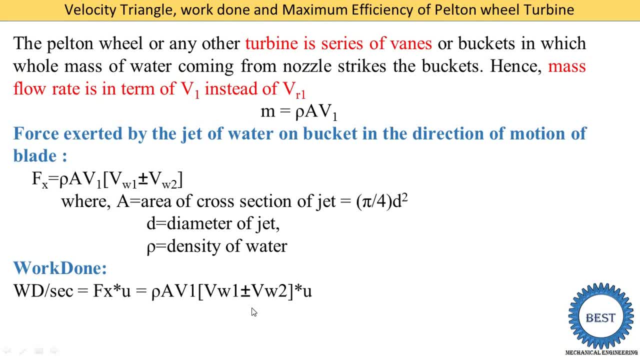 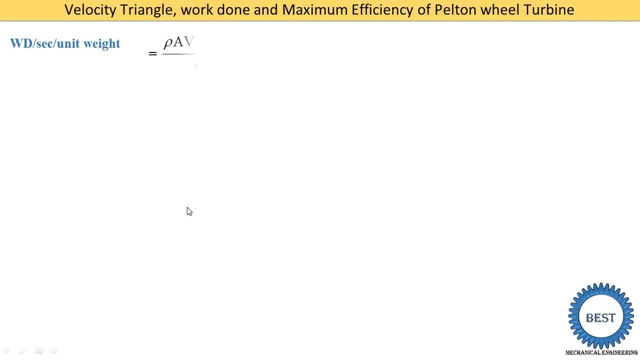 equation of fx, that is, rho a v1 into vw1 plus 1 minus vw2 into, multiplied with this view, then we get the work done. next is work done per unit weight. that is not necessary for deriving this equation, but it is just simply written here. 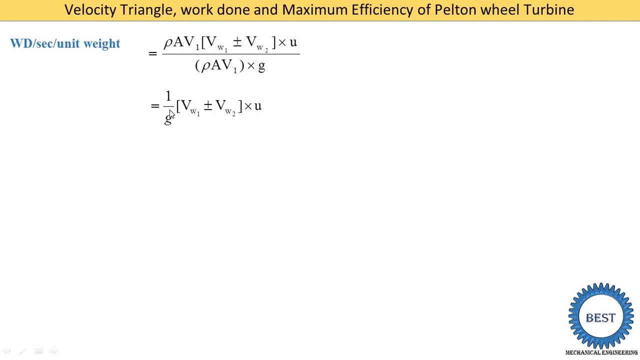 so it is divided by the weight. so weight is equal to rho a, v1 into g and we get this equation now. next we find out the kinetic energy of a jet per second, kinetic energy for a jet. it's considered as 1 by 2 into m, into. 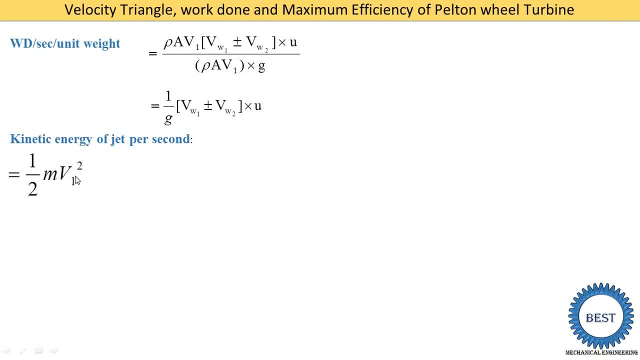 velocity square. so it is a 1 by 2 m v1 square. what is the m that we already written? that is a rho a v1, so that is a 1 by 2 rho a v1 into v1 square. so it is a 1 by 2 rho a v1 cube. so this is the. 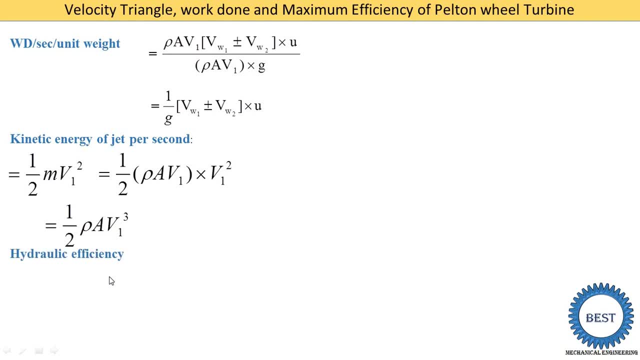 equation for kinetic energy. next we find out the hydraulic efficiency. hydraulic efficiency is equal to work done divided by kinetic energy. so work done. that we already know that is work done per second. that is a rho, a v1 into vw1 plus 1 minus vw2 into u2, that is: 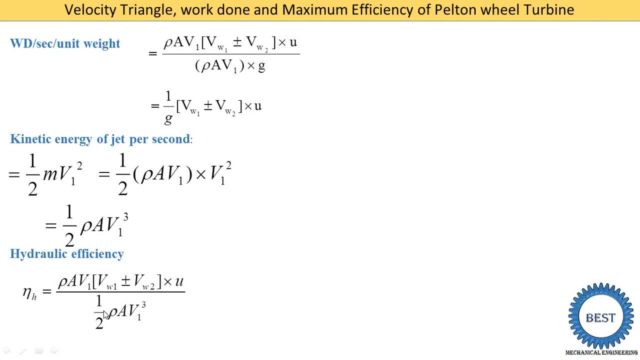 divided by the kinetic energy, that is 1 by 2 rho a v cube. on that rho a v1 is cancelled. these two is moving upper part. so it is a 2 into vw1 plus 1 minus vw2 into u2 divided by v1 square. so this: 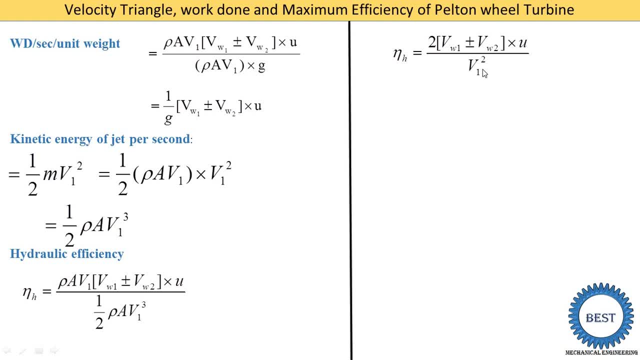 v1, here v1 cube, so v1 is divided and here come is the v1 square. so this is our equation. now, in this equation we putting the value of vw1 and vw2 from a velocity triangle. before that, i request to subscribe my channels, comment on the video, like the video and share with your friends. 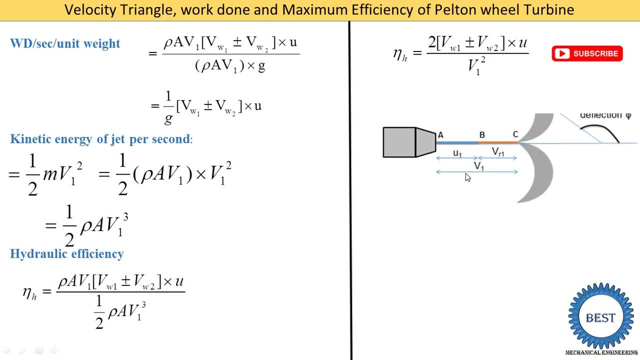 so here i again wrote a velocity line. so in this velocity line this v1 is equal to vw1. okay, that we already learned. so instance of this vw1 we putting the v1 and the vr1 is equal to v1 minus u is equal to vr2. that we conclude from inlet velocity triangle. here again i draw to the outlet velocity. 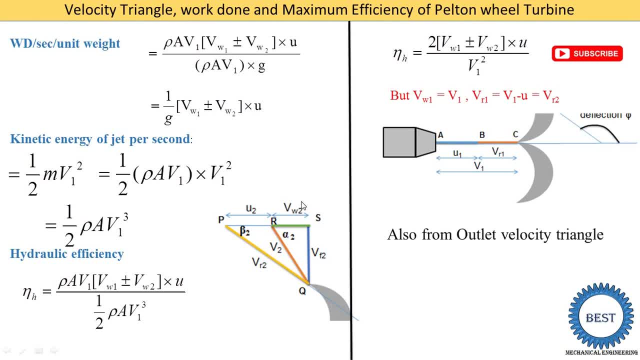 triangle. so from outlet velocity triangle we need to define the value of vw2. for that we apply the of cos, beta 2. cos beta 2 is equal to adjacent side, adjacent side. so we are considered a triangle. pqs so adjacent side is u2 plus vw2. divided by hypotenuse that is vr2. so it is equation is: 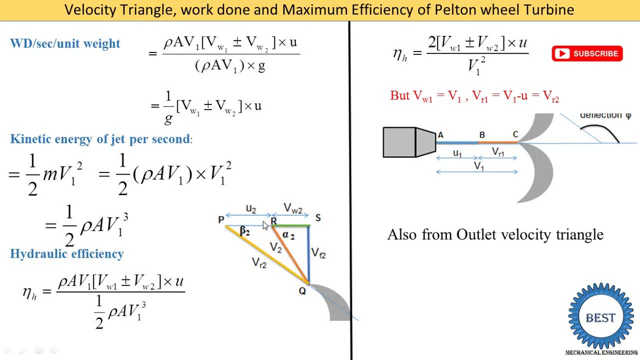 cos beta 2 equal to u2 plus vw2 divided by vr2 and we need to find out the vw2, so it is a cos beta 2 into vr2 equal to u2 plus vw2. so vw2 is equal to vr2 into cos beta 2 minus. 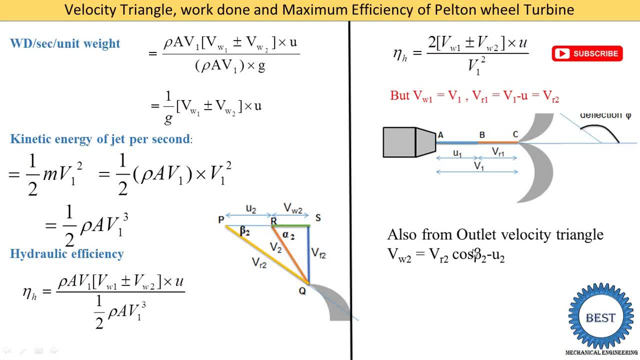 u2. now in this equation we put the value of vr2, so from the inlet vr2 is equal to vr1. so here we write down: vr1 cos beta 2 instance of u2. we write the u now instance of vr1. again we return that is a v1 minus u. so vw2 is equal to v1 minus u. 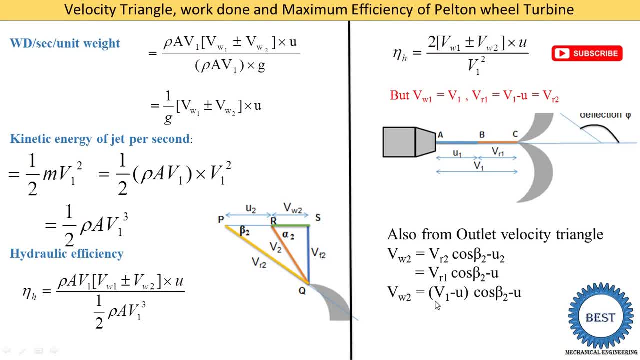 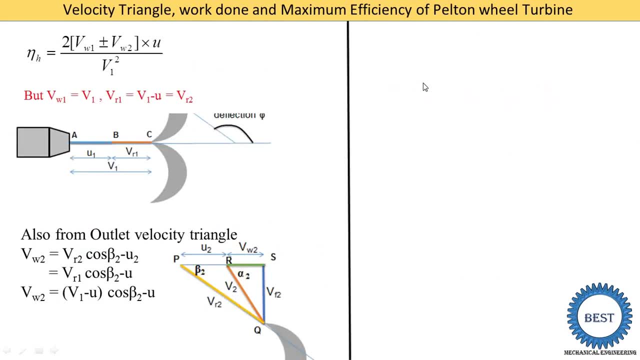 cos beta 2 minus u. now this value of vw1 and vw2 is putting in this equation and we get our final equation. so i just shift this thing on the left side now putting this value in this equation of hydraulic efficiency. so, instance of this vw1, we return v1. instance of vw2, it is written v1 minus. 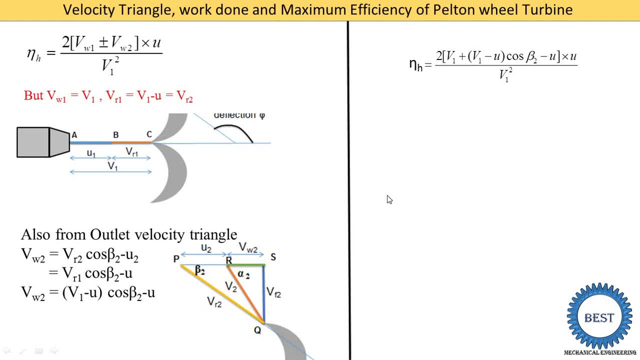 u into cos beta 2 and minus u. now in the next step this v1 minus u is written together, so this minus u is come with this v1, so here written v1 minus u. after that we take the common, that is, the v1 minus u is taken common, then this step is written like this way: 2: 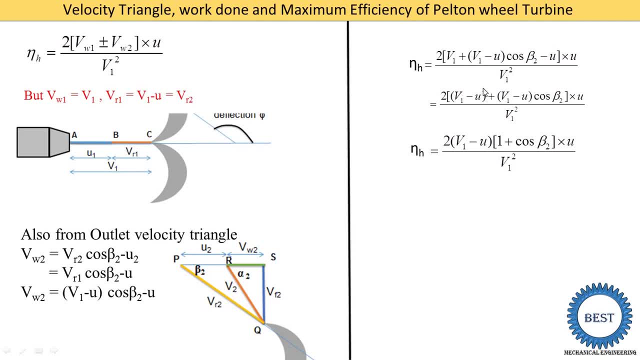 into v1 minus u is common. so in bracket instance of this v1 minus u, it is a 1 plus this going and is the cos beta 2 bracket over into u divided by v1 square. now this is our final equations for hydraulic efficiency. 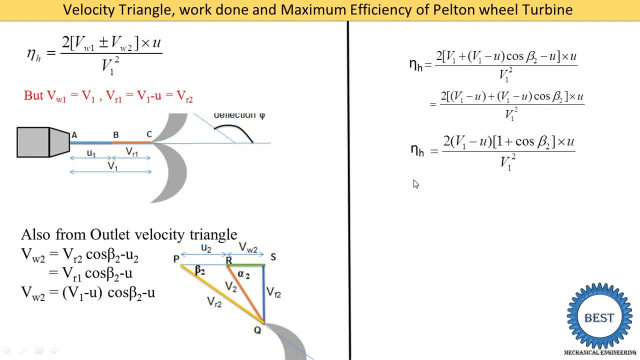 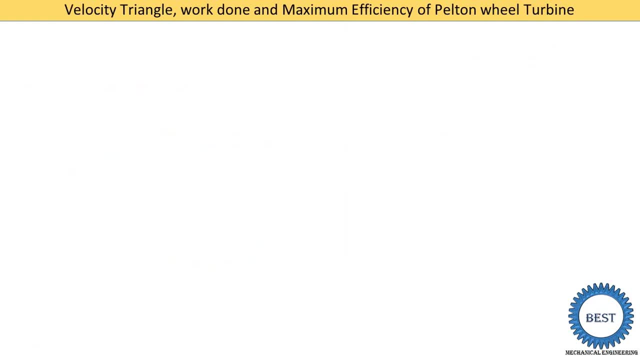 next we will study maximum efficiency for a pelton wheel turbine or finding out maximum efficiency. we need to derive the condition for maximum efficiency. so first we find out condition for maximum efficiency. for that we need to differentiate this equation with the velocity u, so this equation is differentiate with the u, so the constant parameter, we take the common. 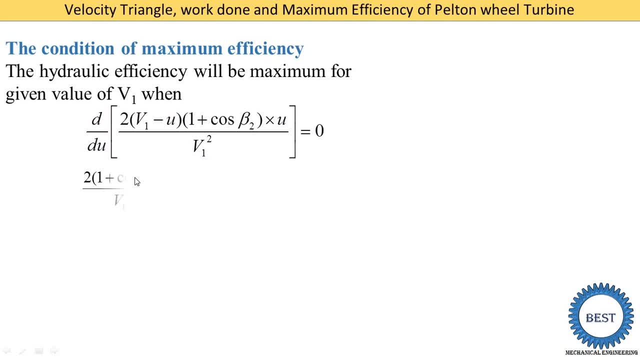 that is the 1 plus cos beta 2 upon v1 square is coming the common, because they are not doing the common differential. so only we differentiate, that is a v1 minus u into u square. so here we open the bracket v1 minus u into u, so it is v1 minus u into u into u u square. so for during: 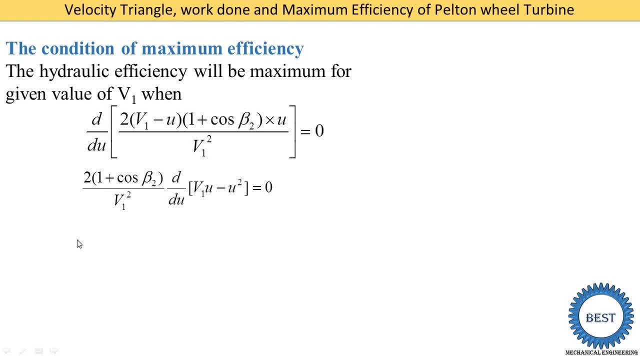 for that we need to differentiate only by using the simple equation that suppose x raise to n power, then n is come forward into x raise to n minus 1. so in this our case, u is our x and the power is 1, so 1 is come ahead, and 1 minus 1, that is a 0, so u is equal to 1 in. 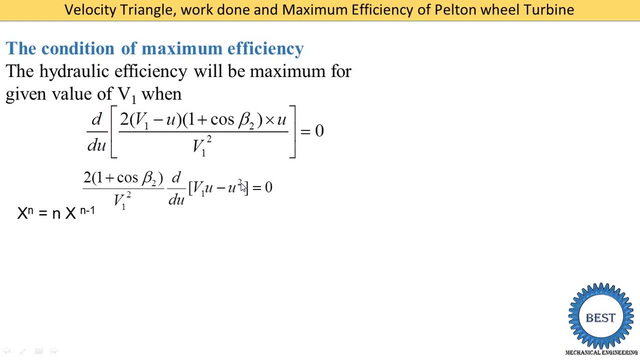 this case, x is u, power is n is equal to 2, so 2 is coming forward. u raise to 2 minus 1, that is a 1, so it is a 2 u. so this differential is written like that: v1 minus 2, u is equal. 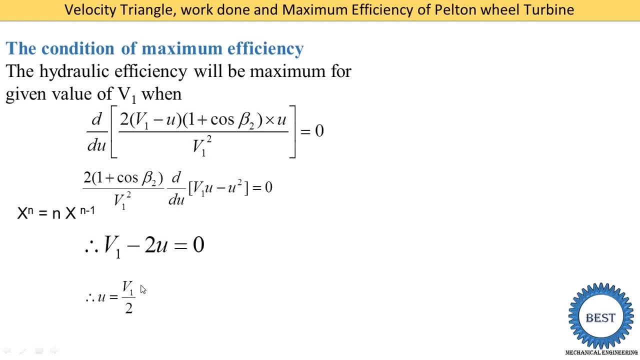 to 0. for that we finally conclude that u is equal to v1 by 2.. now this is our condition for maximum efficiency. if we achieve this condition, then we are able to achieve a maximum efficiency. now we are putting this value of u is equal to v1 by 2 into equation. 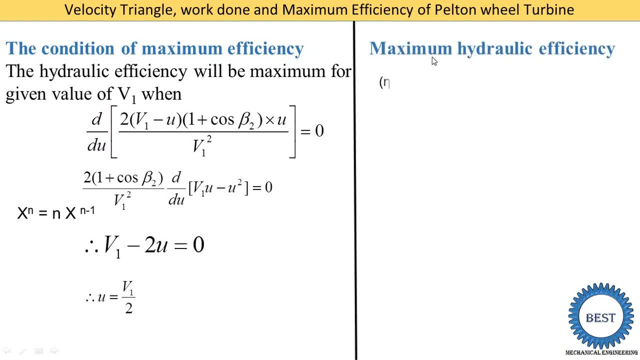 of hydraulic efficiency. so here i again written the equation of hydraulic efficiency. now this efficiency is known as maximum. so here we need to write down m, a, x. now instance of u. we are putting v1 by 2 in this equation of hydraulic efficiency, so all the u is replaced. 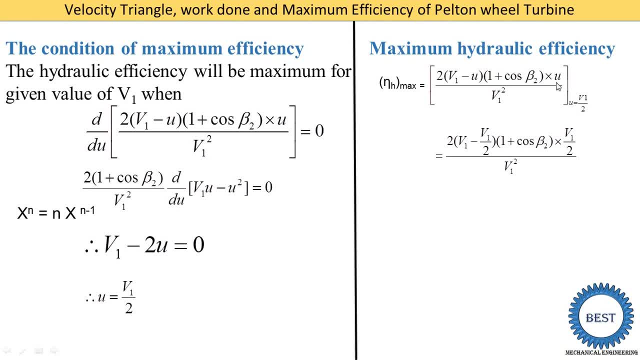 by v1 by 2. so here u it is replaced by v1 by 2. this u is also replaced by v1 by 2. now we simplified it. after simplifications we get the final equation, that is 1 plus cos beta by 2. so this is the final equations for a maximum efficiency. and from this equation 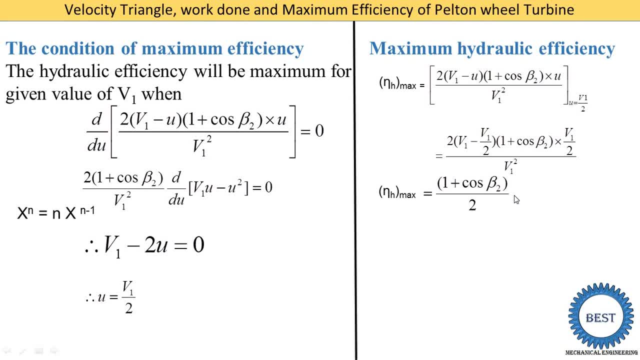 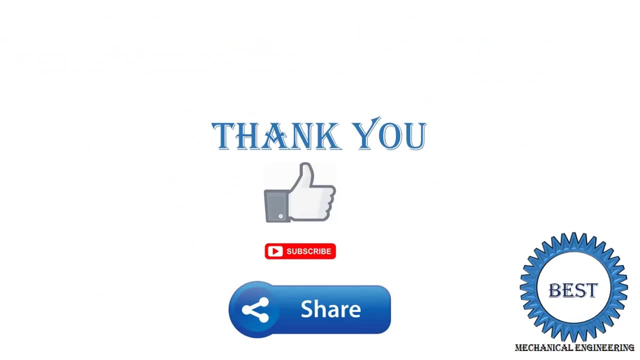 we conclude that maximum efficiency for a pelton wheel turbine is only depend on a blade angle, beta 2.. not depend on the any velocity of a pelton wheel turbine. it is only depend on the beta 2.. thank you for watching this video. if you learn something, then like my video, subscribe my channels and share with your friends.